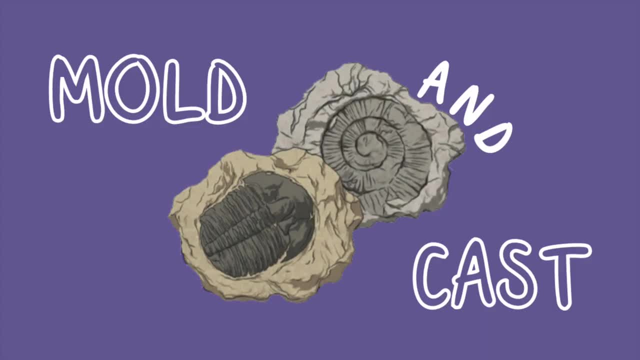 Body Fossils. After an animal or plant dies, all of the parts of the body decay. The skeleton is covered by layers of rock. Eventually, the bones of the skeleton also break down, leaving an empty space in the shape of the animal or plant called a mold fossil. 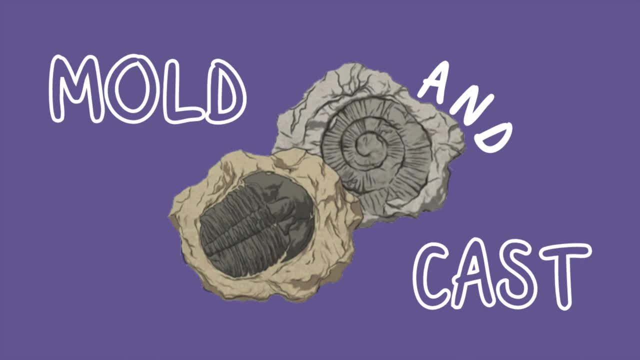 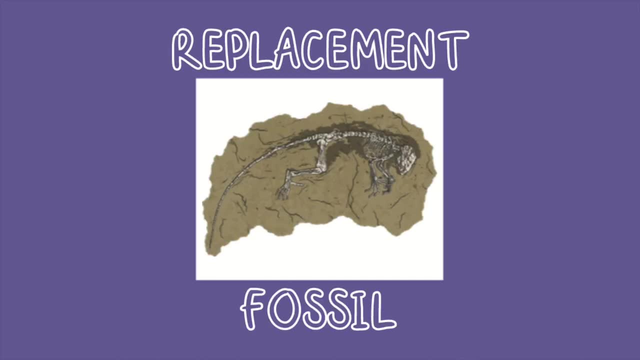 This empty space can then be filled with sediment which hardens, creating a cast fossil. Sometimes, only the soft parts inside the bones decay, leaving the hard outside of the skeleton. The bones have small holes in them, like a sponge, which can fill with minerals. 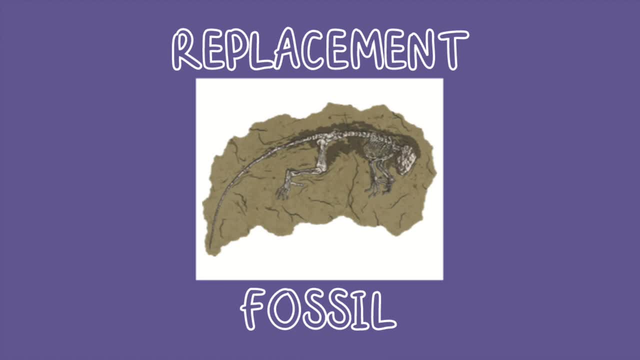 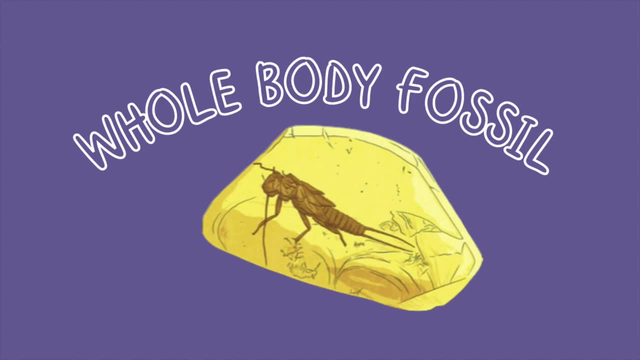 The minerals then harden. This creates a replacement fossil Whole Body Fossils. Whole body fossils are formed when an animal or plant is preserved in ice or peat bogs or trapped in fossilized tree resin such as amber. Whole body fossils are formed when an animal or plant is preserved in ice or peat bogs or trapped in fossilized tree resin such as amber. 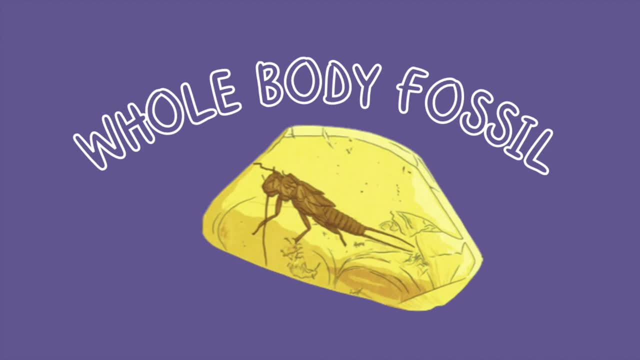 Whole body. fossils are formed when an animal or plant is preserved in ice or peat bogs or trapped in fossilized tree resin such as amber. They do not decay at all and look exactly like they did when the animal or plant died. 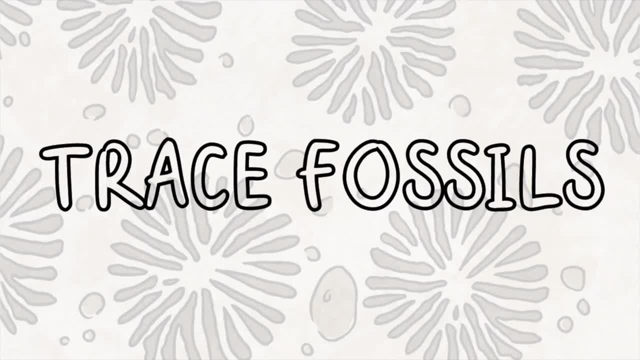 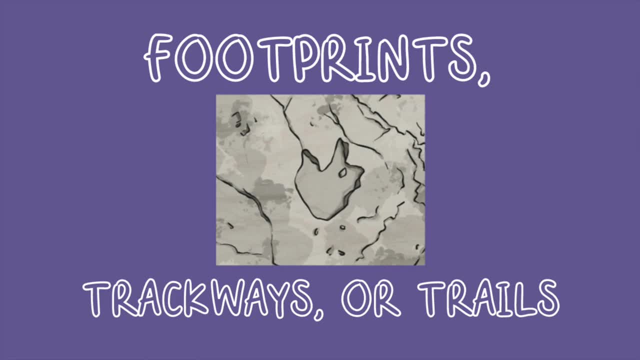 Whole body. fossils are formed when an animal or plant is preserved in ice or peat bogs or trapped in fossilized tree resin, such as amber Trace Fossils, Trace Fossils, Footprints, trackways or trails that show the movement of an animal. 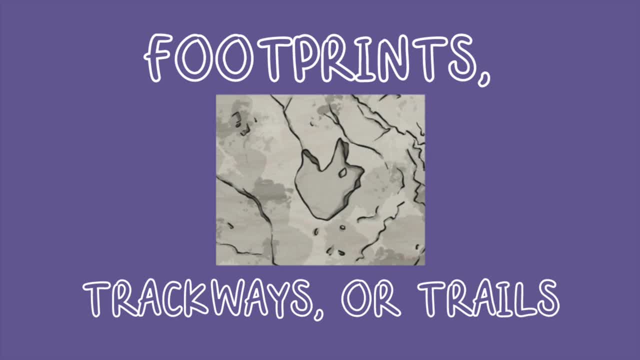 The fossilized footprints or trails are made. when the animal makes an imprint in mud or sand, which then dries and hardens, It is covered by new layers of sediment which also harden to rock, and the footprints are preserved. Fossilized Burrows. 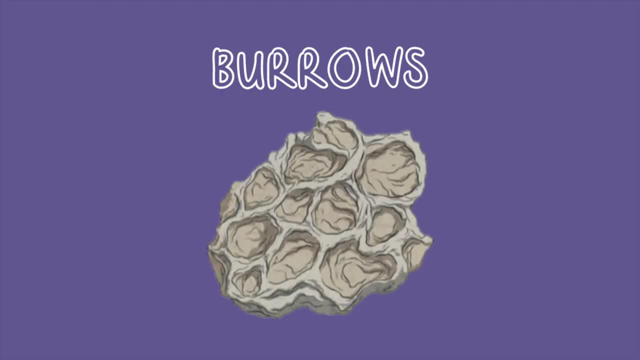 Fossilized burrows or borings can be made in a similar way to footprints and trackways. The animal makes the markings by digging or burrowing into sand or mud. Animal feces that has become fossilized is known as coprolite. 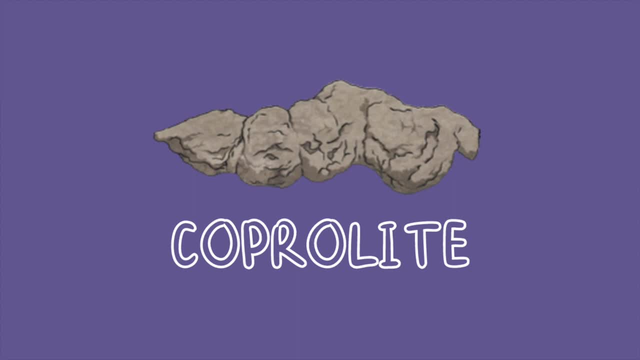 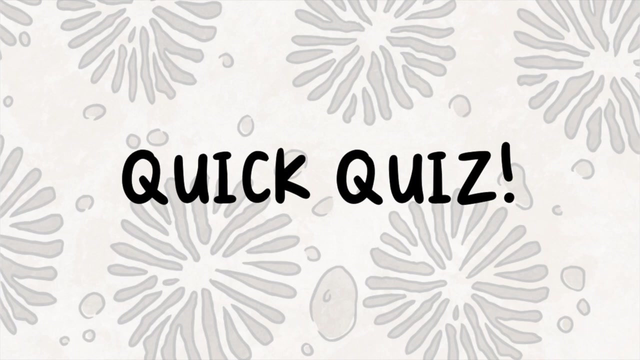 Scientists can study it to work out what animal it might have come from and what that animal might have eaten. Fossilized Burrows and Trackways, For example. evidence of bone would suggest that the animal was a carnivore. Quick Quiz: Fossilized Burrows and Trackways.